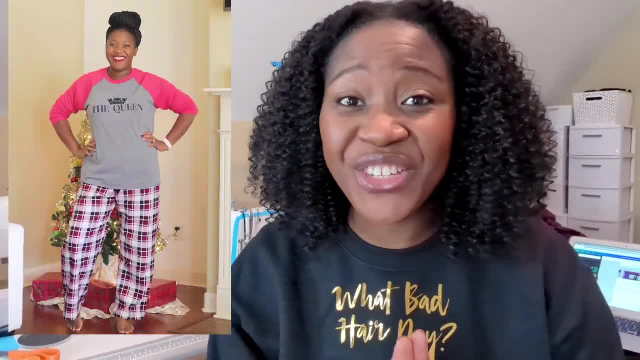 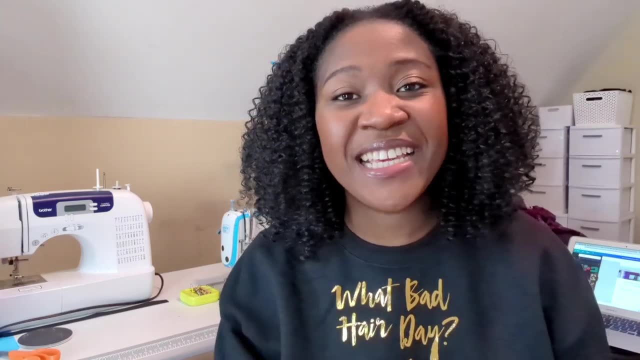 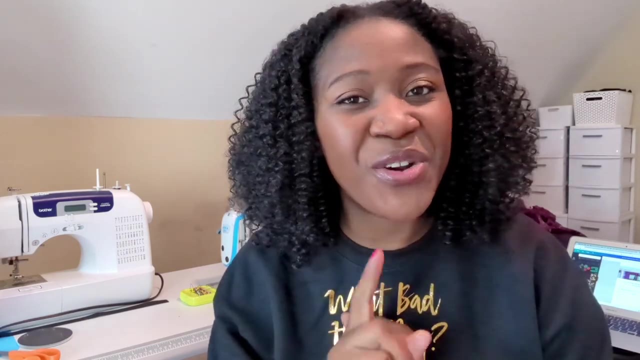 These are going to be a bit more complex, but still, all you need to do is know how to sew in a straight line, know how to hem. The only hard part here is cutting out the pattern for the pants to be able to fit you, because if you do not cut these correctly, there's a chance that these 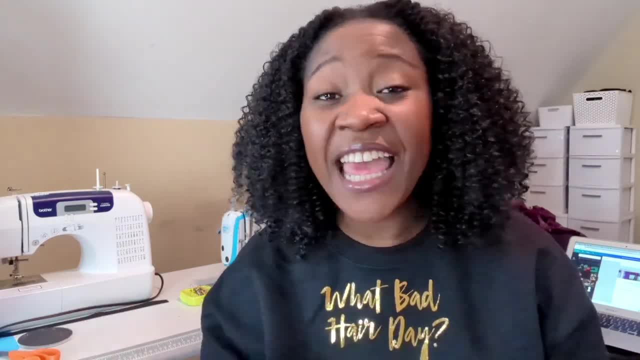 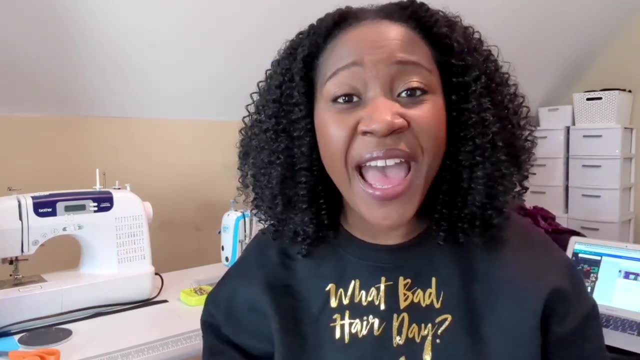 pants might not fit you. So that's the only complex thing. Like the elastic waist skirt, all you need to do is make an encasing, put in the elastic and voila, you have those pajama pants. Number three is a kimono duster. Now, I know there's a bit of 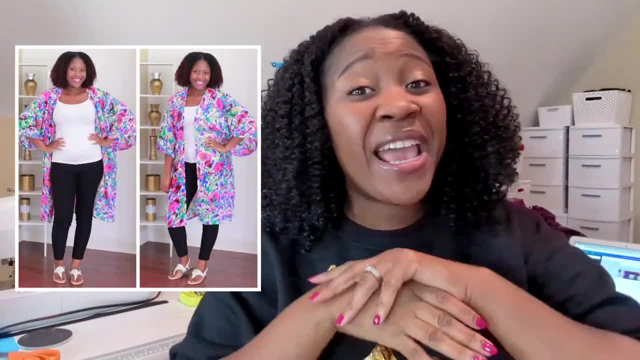 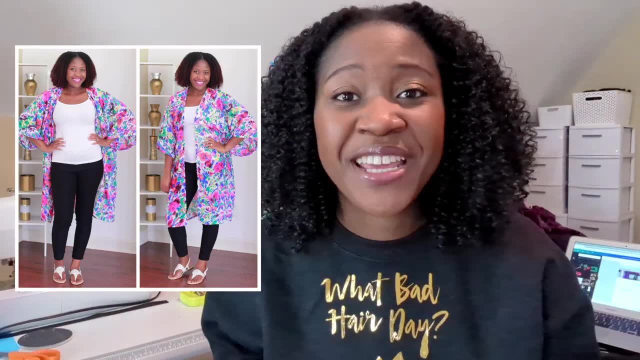 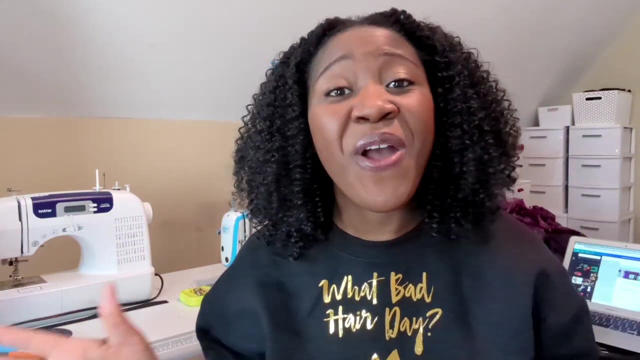 controversy about the word kimono and I apologize if that's not the right word that I should be using, but let's say kimono-inspired duster. Super easy Again. the most complex part of this sewing project is just cutting out the shape of the kimono. but, like I said again, if you can do, 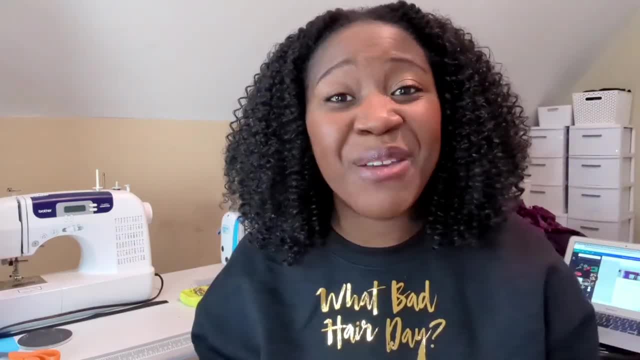 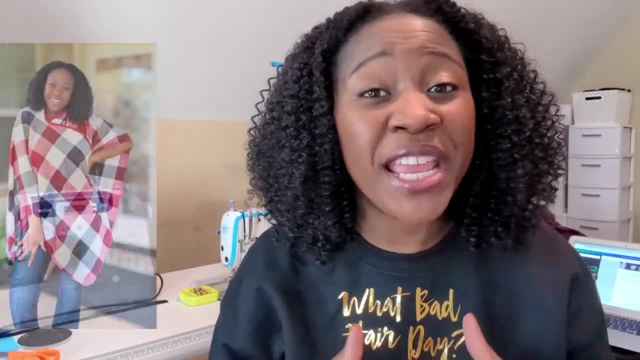 a straight line, a straight stitch, you can make a kimono duster. So number three is a kimono jacket or duster. Number four: a cape or a poncho. I have a no-sew version for a cape or a poncho. 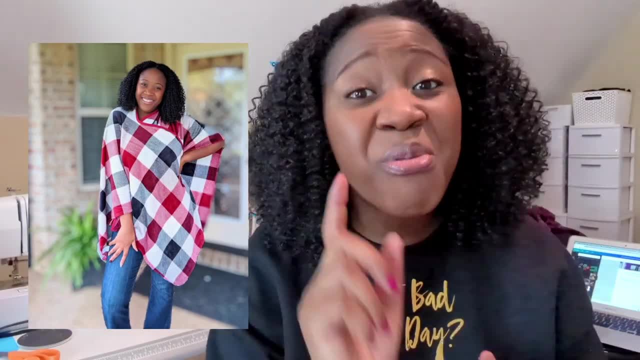 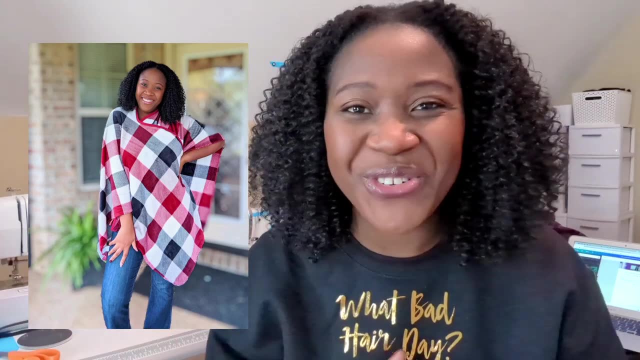 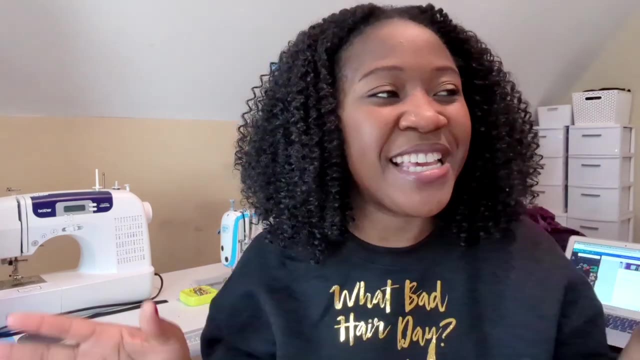 but we want to learn how to sew, So I suggest that you practice actually sewing, or the sewing version of this, and super easy Again. all you need to do is know how to sew a straight stitch. sew some binding onto your cape and you have a cape Super easy. I think this is like the easiest. 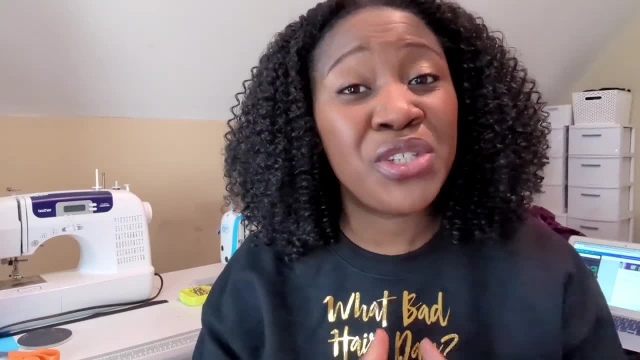 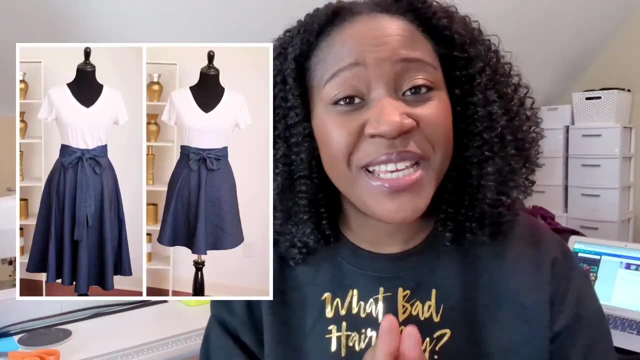 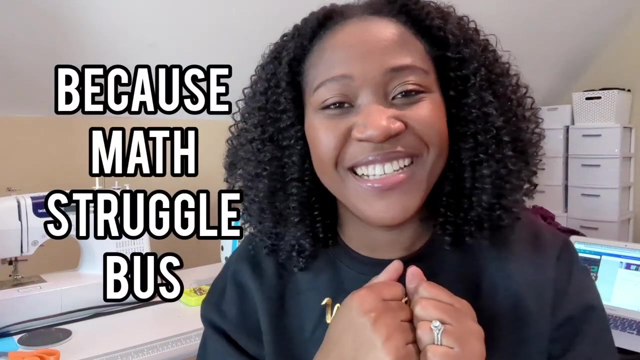 project that you can do. Number five is a circle skirt. Now, for this one you will need kind of like circumference measurements and, oh my gosh, already like confusion. but not to worry, I don't even make calculations for this, So what I actually do is just take my waist measurement. 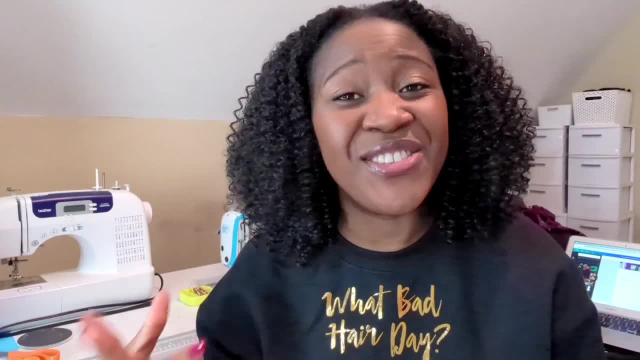 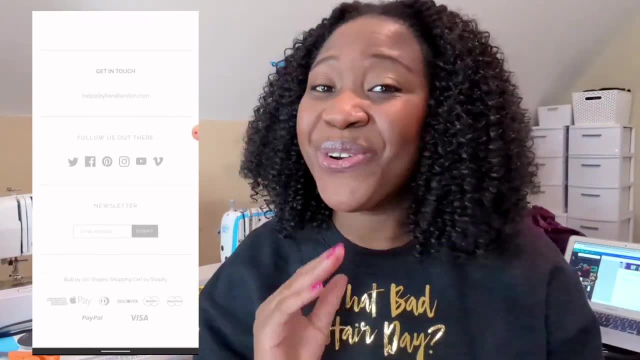 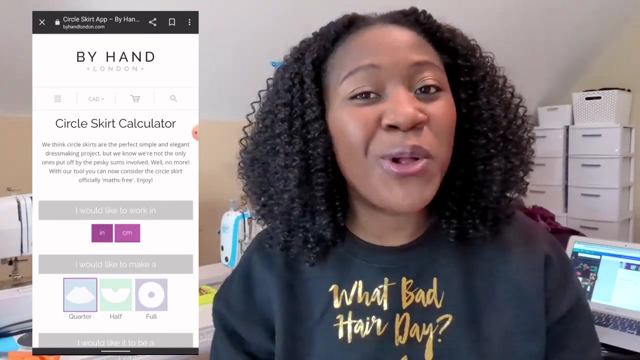 and there's a handy-dandy app. This is not sponsored, This is not an affiliate and I pray that these guys never take that. I have been using their site for years, So all you do is take your waist measurement, put them into this handy-dandy app that they have and the name of the website is called By Hand. 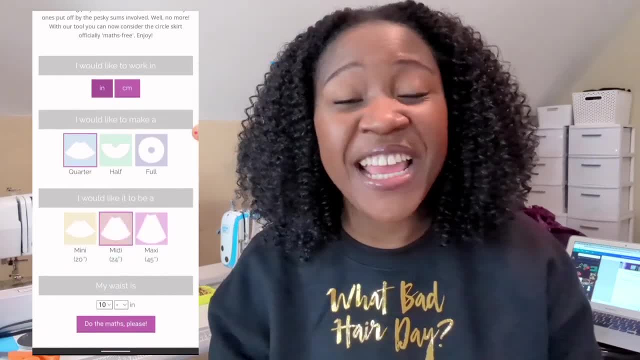 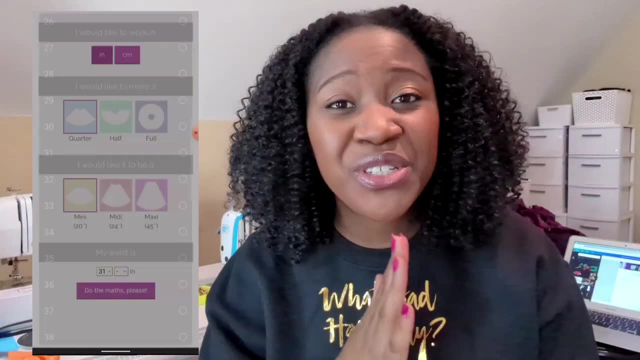 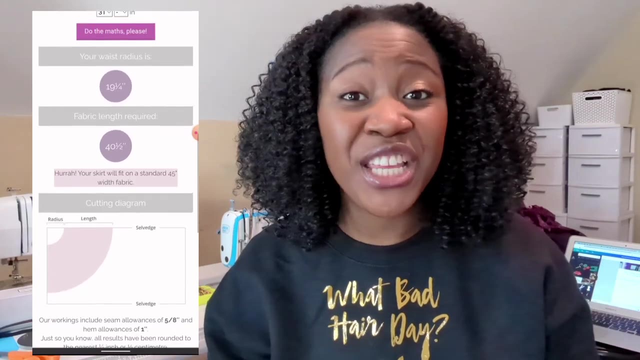 London and you can just put in By Hand London Circle Skirt and it gives you all the calculations that you need to make a circle skirt. They even show you how to cut out your fabric, how much fabric that you need, and so, oh my gosh, once that is done, you are set, You are ready to. 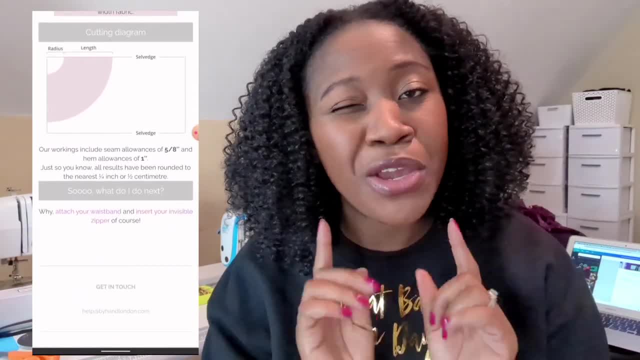 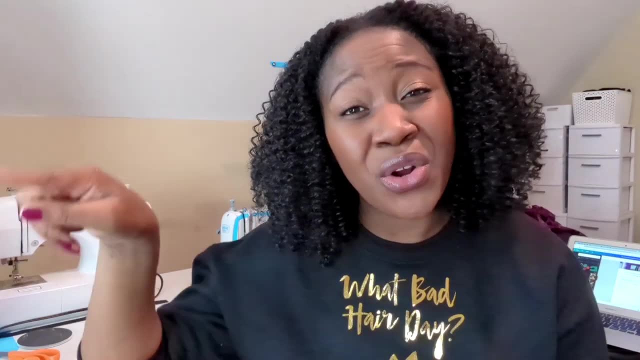 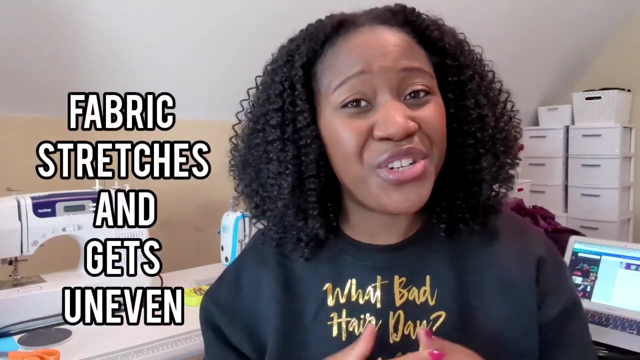 sew your circle skirt. Now, with the circle skirt, the only challenge would be the hem, because even though it's a straight line, it is mostly going to be in a circular kind of like, in a circular motion, and so sometimes fabric can act funny whilst you're sewing and your hem might come out a. 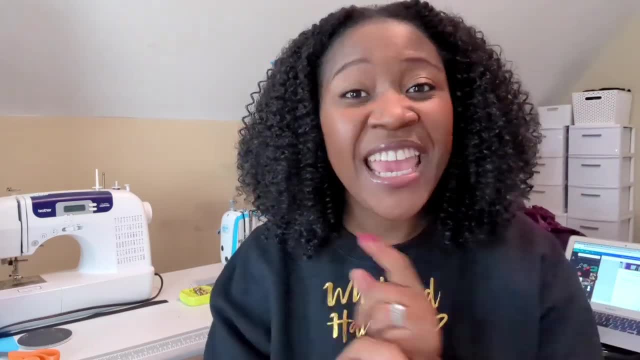 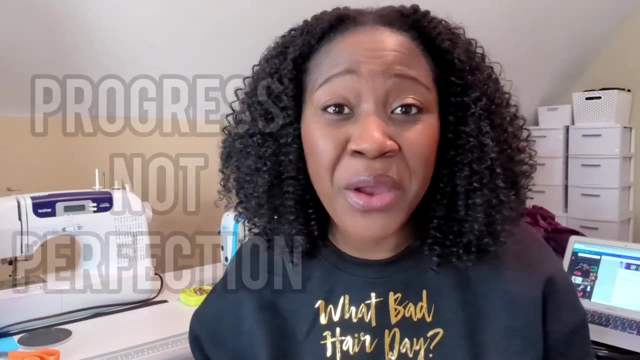 little crooked. but hey, practice, Keep practicing. It doesn't have to be perfect the first time. My stuff like to me, it's fine. I'm sure if someone came and inspected what I was doing they would think, oh my gosh, that's not perfect. but anyways, listen. 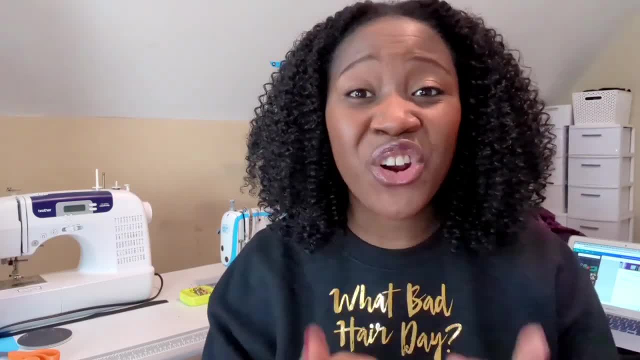 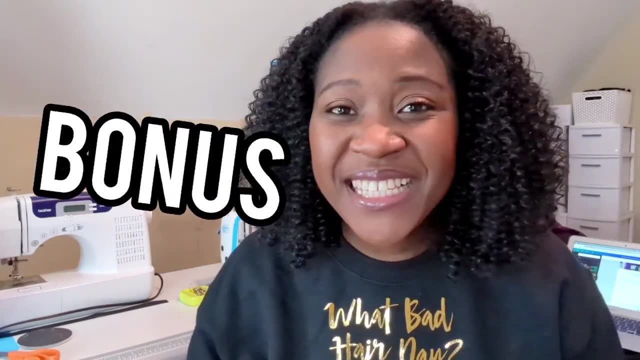 as long as it's good for me, it's good. So, yes, a circle skirt. it is beginner, but slightly, slightly advanced. and a bonus project that you could make is Palazzo Palooza, Palooza. 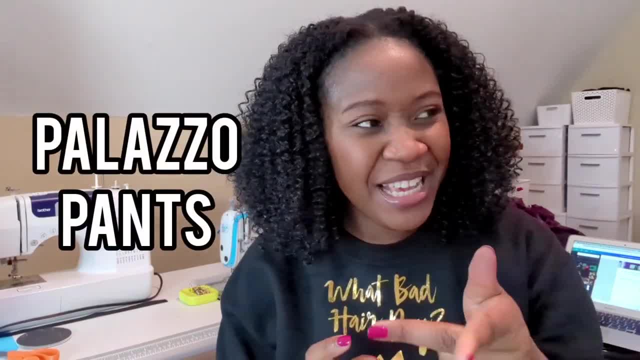 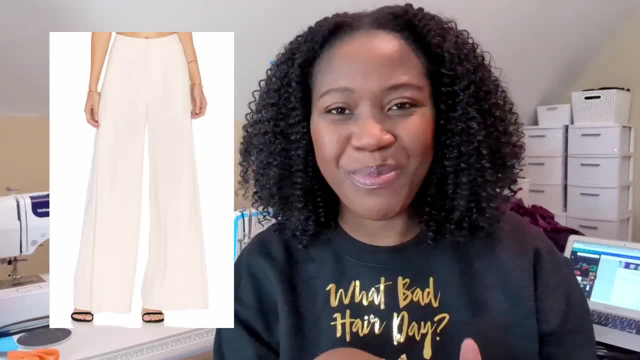 Palooza pants- Palazzo pants. I call them Palooza pants. Let me know in the comments what the right or the correct pronunciation is. I'm going to give you a few examples. It's a really good, really fun project. I don't even know. 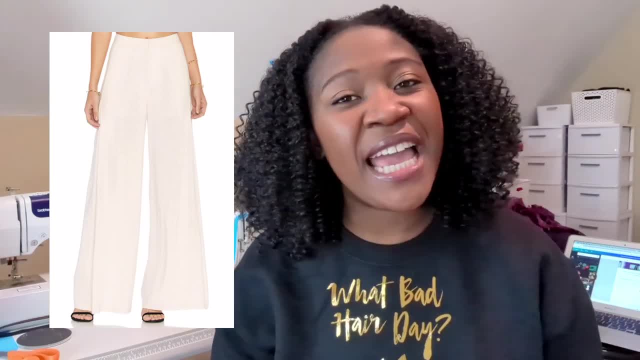 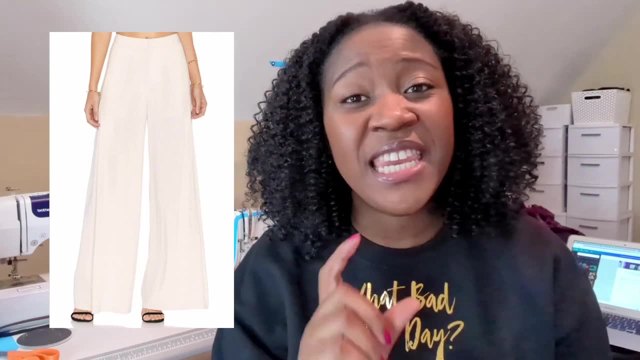 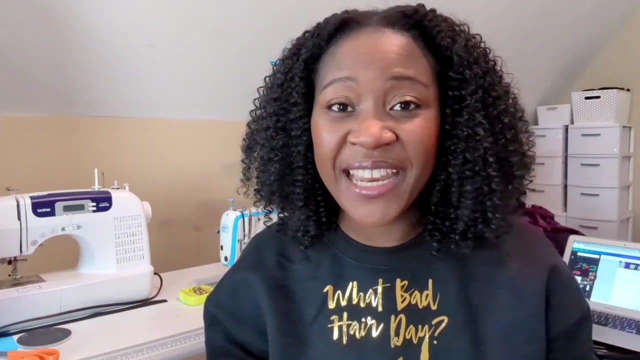 what the right pronunciation is for those pants, but they are just like knit, very stretchy pants, so they're almost like pajama pants. Pajama pants would be made out of woven fabric, but for these you'll be making them out of knit fabric, and I don't think they have an elastic waistband. They 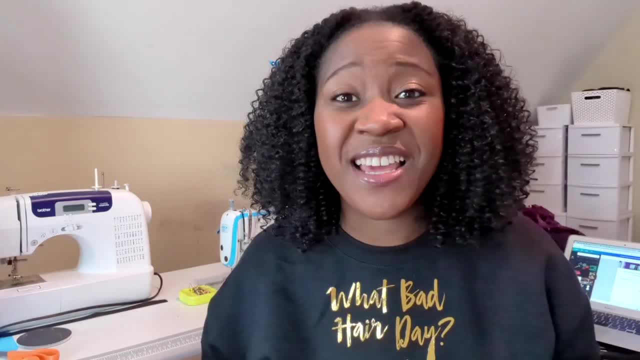 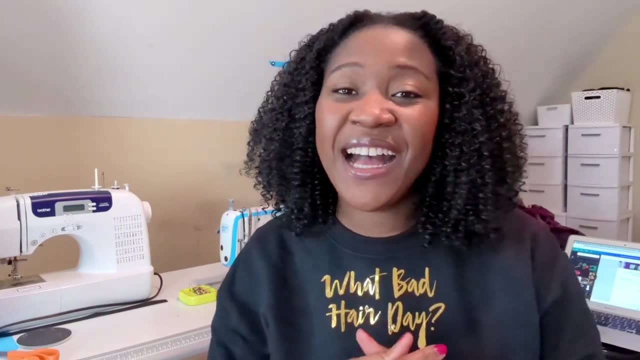 just have like a stretchy waistband which is supposed to keep the pants up and be snug enough. so this is another easy project that you would be able to make, to do and where. So those are all the projects that I have. For each of these projects, I will 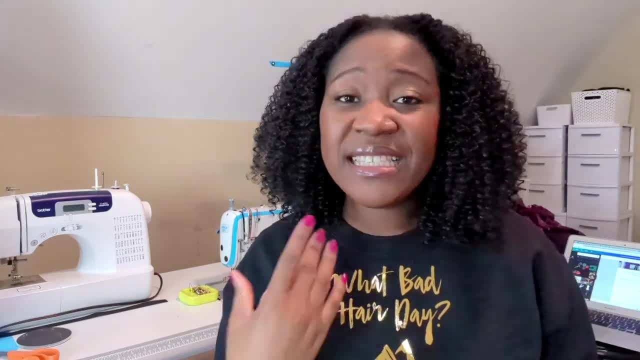 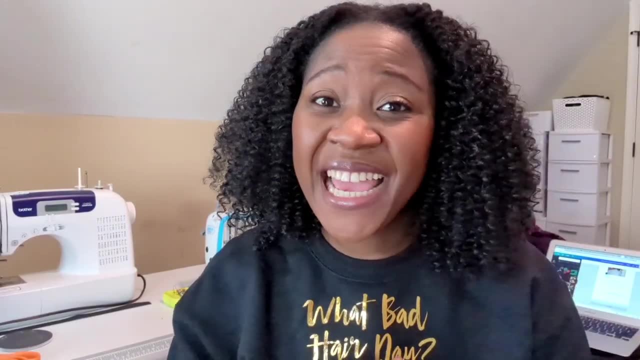 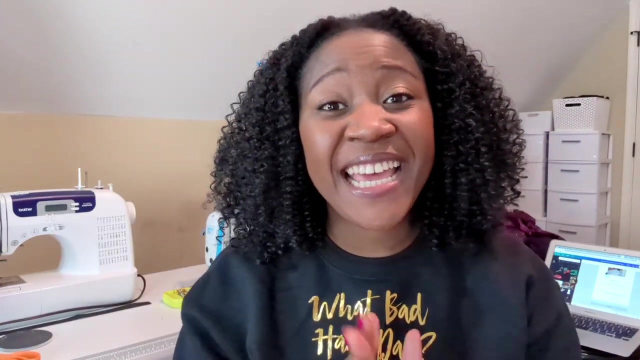 link a video where you can actually see how you can make these things so you can try and practice. I'll link all of those in the description box. I will also provide a download and that will be in the description box as well- A download just listing all of these projects that I have.